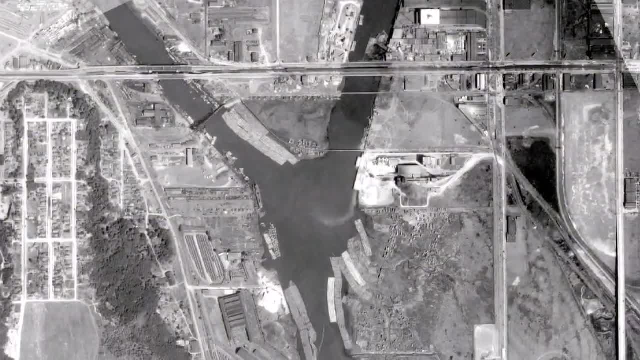 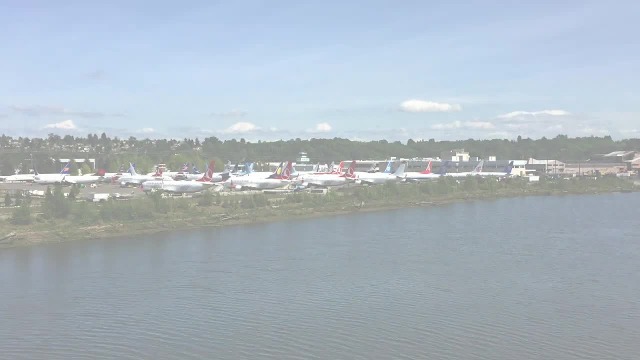 into a straight channel or waterway for ships and industry. Through World War I and World War II, Seattle's population and industries boomed. Raw sewage and wastes from airplane manufacturing, shipbuilding, metals, recycling and other industries were poured into the river. 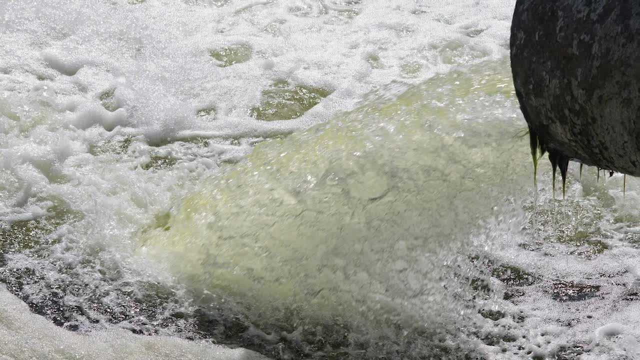 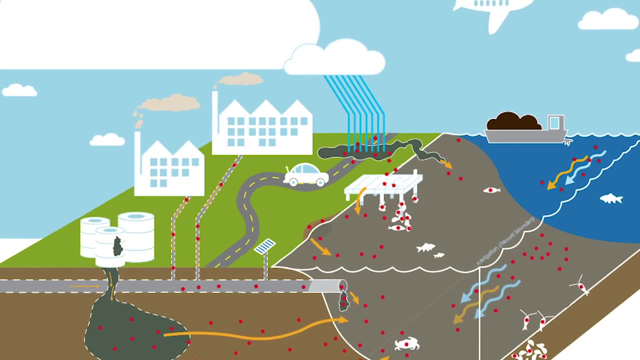 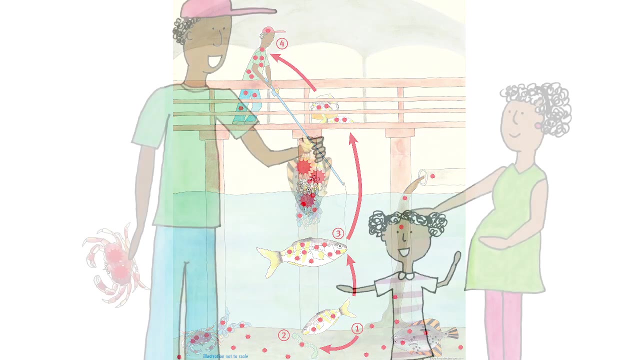 This waste was full of pollutants and settled into the mud or sediment of the river bottom. When these pollutants get into the river sediment, they are picked up by worms and other creatures, Which are then eaten by fish and other wildlife. People can be exposed to these pollutants when they come into contact with polluted mud while clamming. 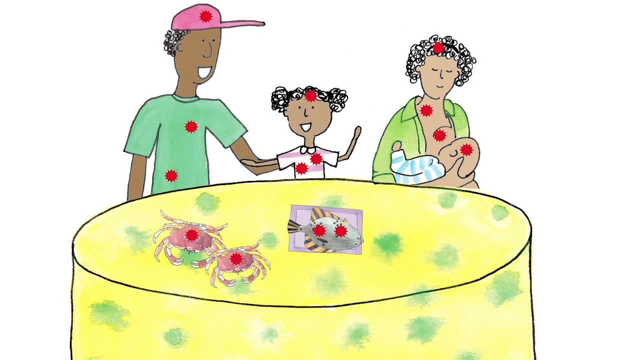 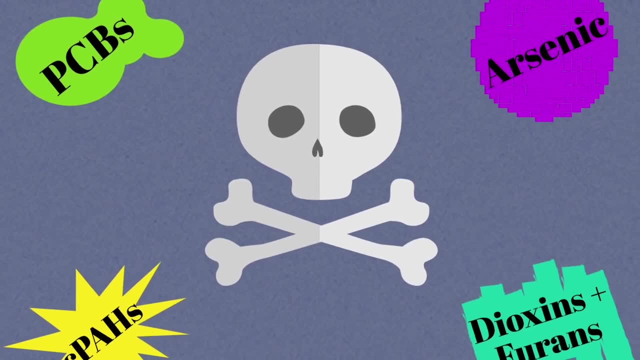 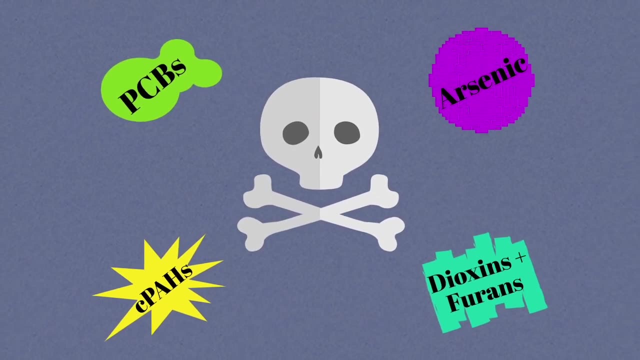 but the biggest risk to people is when they eat polluted resident fish. Pollutants in the fish include polychlorinated biphenyls, or PCBs, arsenic, carcinogenic polycyclic aromatic hydrocarbons or CPAHs, dioxins and furans. 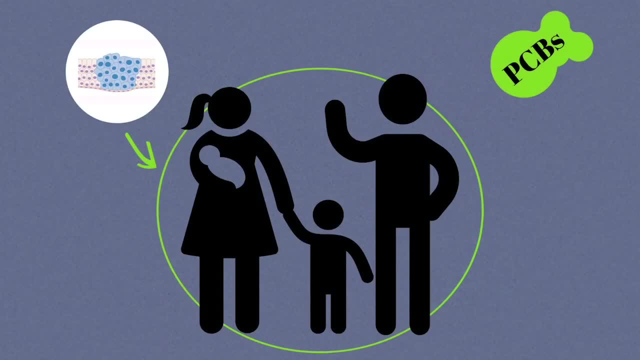 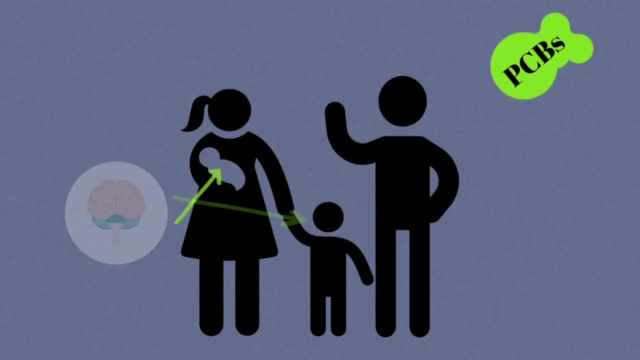 PCBs are the most common pollutants in the river. PCBs may cause cancer in people who have been exposed to them over a long time. They can also affect learning abilities in children. PCBs are linked to other adverse health effects, such as low birth weight, thyroid disease and immune system disorders. 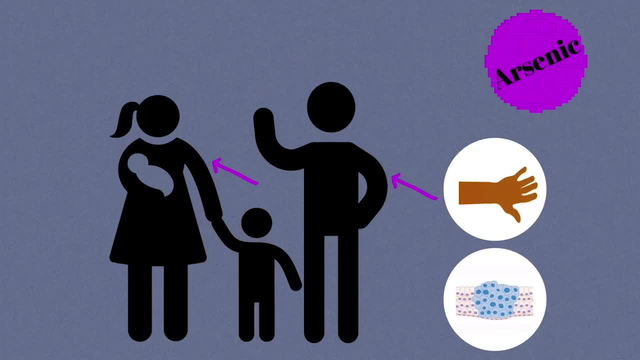 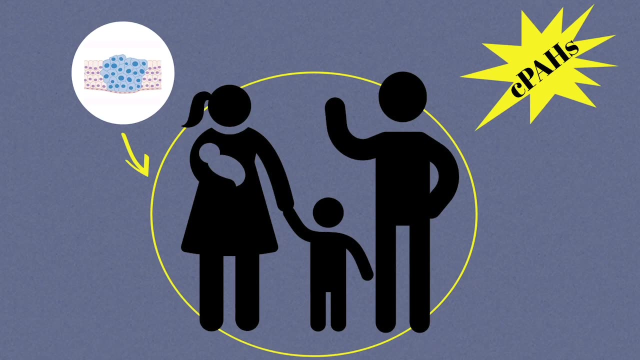 Long-term exposure to toxic forms of arsenic may cause skin, bladder and other cancers. Long periods of breathing, eating or having skin contact with high levels of CPAHs increase a person's risk of cancer. Toxic effects related to dioxins and furans include 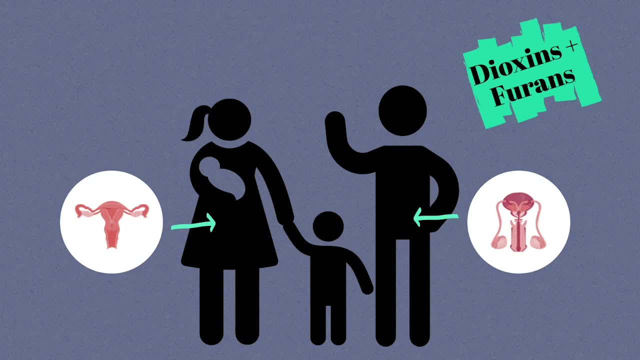 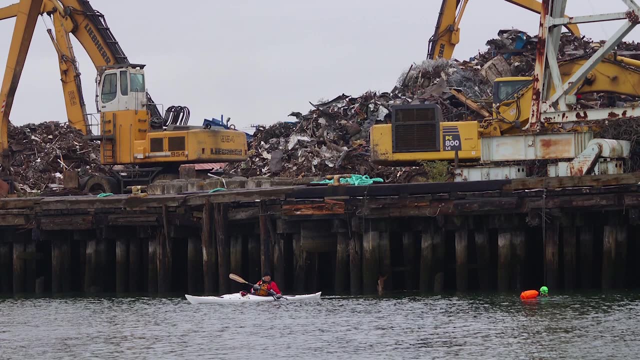 reproductive problems, problems in fetal development and early childhood, immune system damage and cancer. People are still polluting the Duwamish, but not nearly as much as we used to. That's because, as a society, we now know that most pollution doesn't just disappear when it gets dumped in the water. 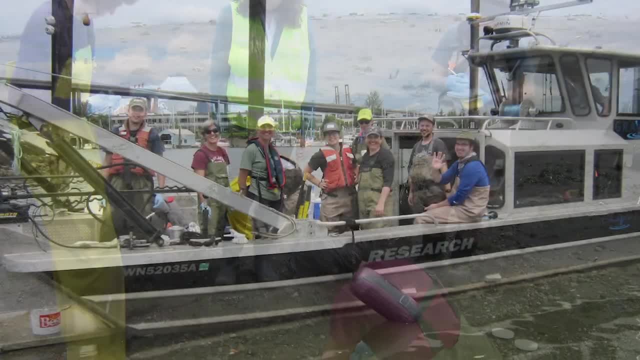 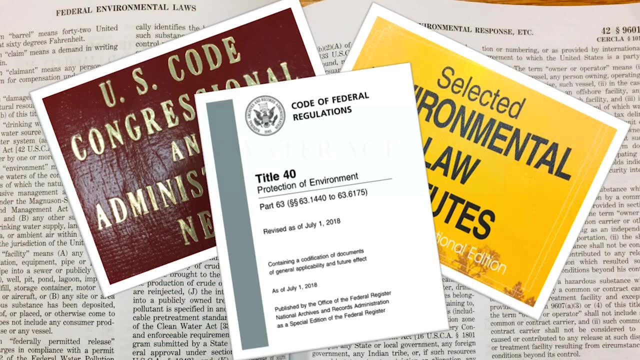 It took us a long time to learn this, but once we did, we understood that we needed to do something about it. Today, there are strict laws that limit the amount of pollution that's allowed to go into the Duwamish or any other body of water. 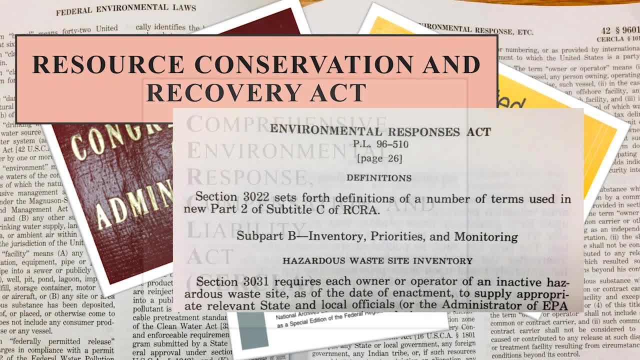 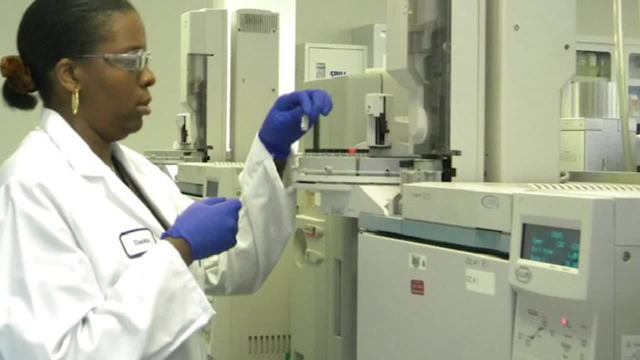 And there are laws to ensure that past pollution is cleaned up as well. One of these laws, called Superfund, requires EPA to identify and clean up the nation's most contaminated sites When deciding if a place should be put on the Superfund list for cleanup. 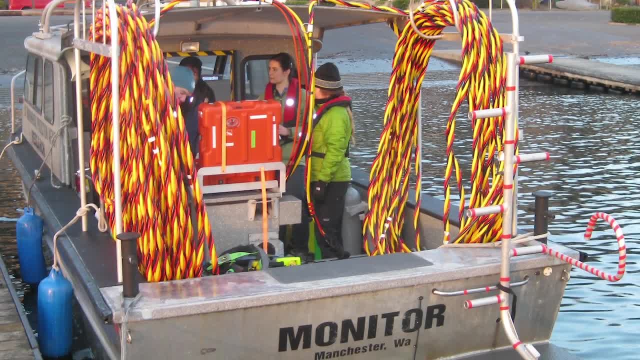 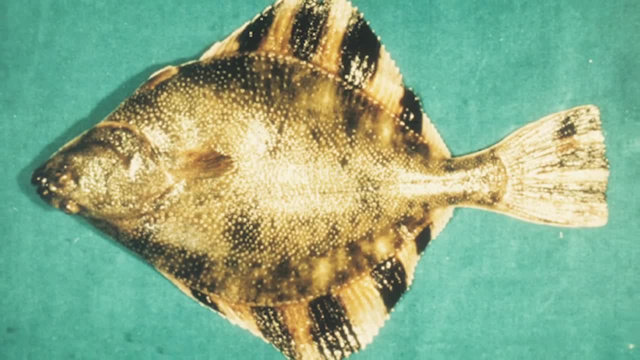 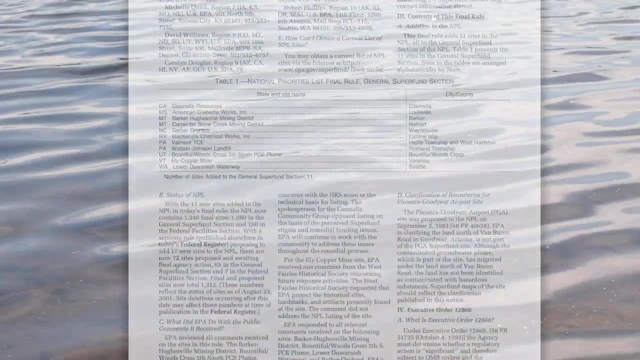 EPA has to find out whether the health of people and the environment are at risk from the pollution. Back in the 1970s, scientists started to find harmful chemicals in Duwamish fish and shellfish. In 2001,, EPA added the lower Duwamish to its Superfund list. 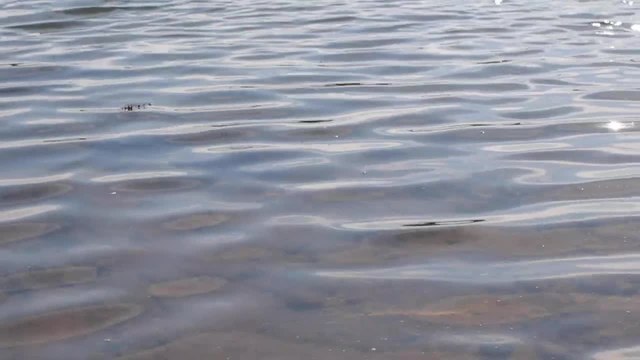 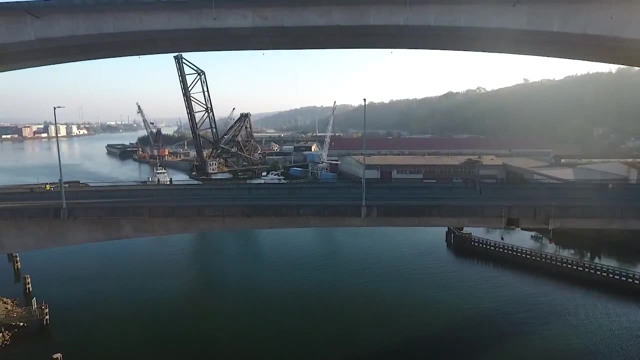 because the number and amount of pollutants in the mud or sediment of the river bottom and in the fish and shellfish that people eat pose a significant risk to people's health and the environment. The Superfund law is based on the principle that the polluter pays. 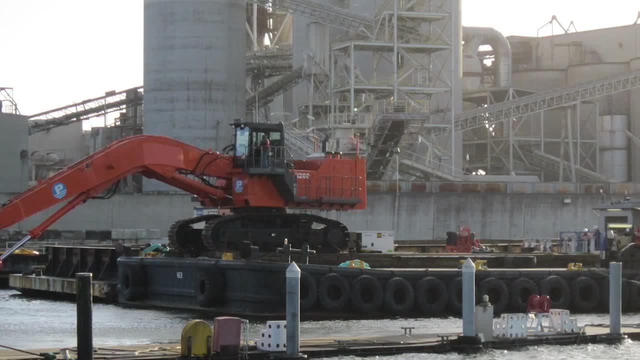 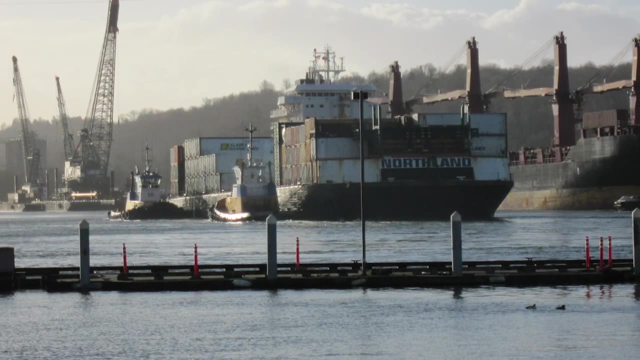 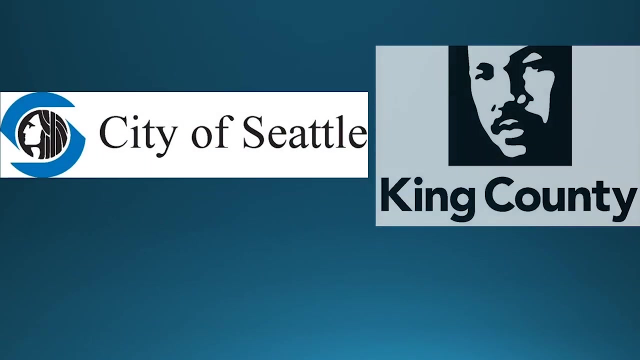 EPA can require responsible parties to clean up the pollution to reduce the risk to people and the environment. In the Duwamish there are many businesses, landowners and local governments who will share in the cost of the cleanup: Four parties, the City of Seattle, King County, the Port of Seattle and Boeing. 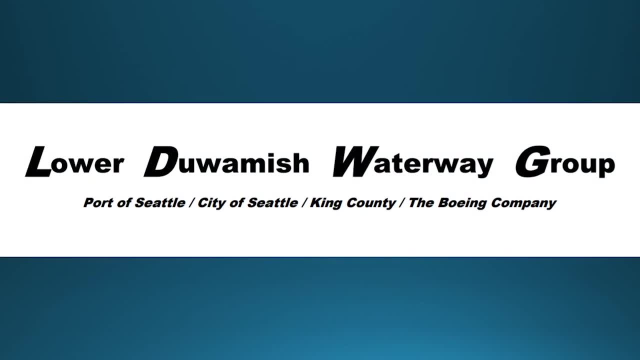 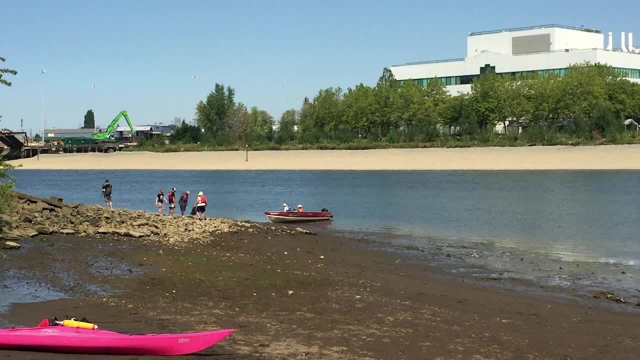 stepped up early on to form the Lower Duwamish Waterway Group. They agreed to study the site and take early actions to clean up some of the worst areas of pollution. Five early action areas were cleaned up while EPA continued to study the Duwamish as a whole. 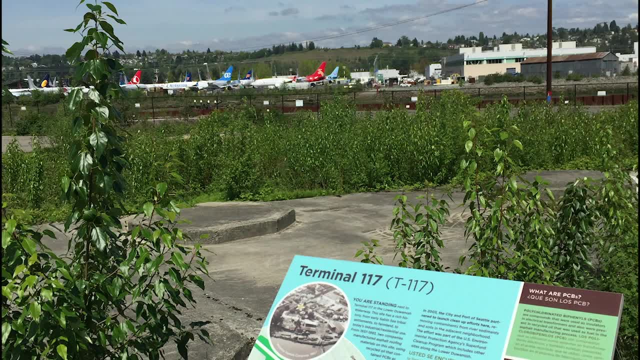 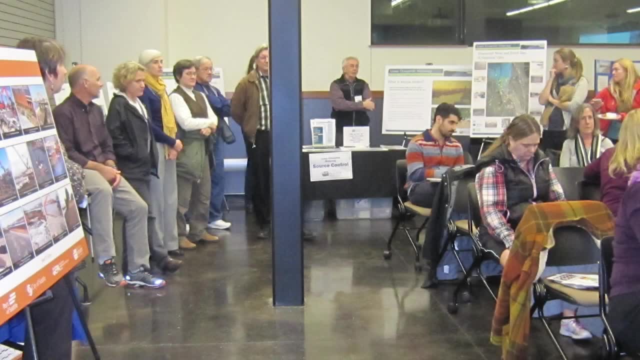 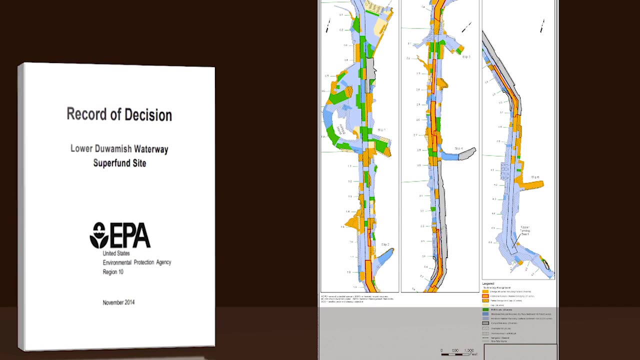 Thanks to these actions, the average level of PCBs throughout the area has been reduced by about half. In 2014,, EPA finalized a plan to clean up remaining areas of polluted river sediment. This final cleanup plan, also known as the Record of Decision or ROD, combines four methods to clean up sediments. 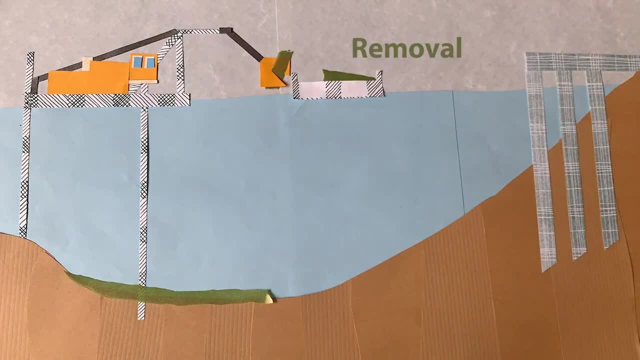 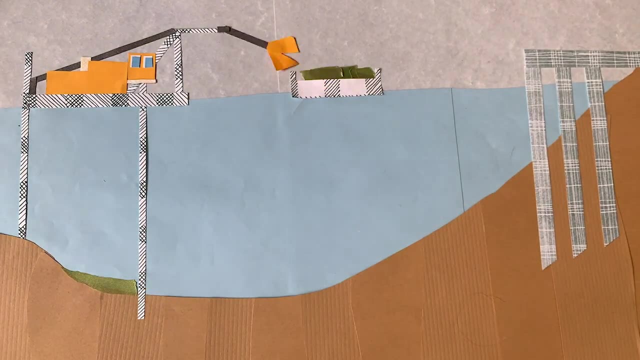 One method is removal or dredging, which means scooping out the pollutants with the sediment and sand it's sitting in. In all, close to a million cubic yards of polluted sediment will be removed or dredged from the river and taken to landfills. 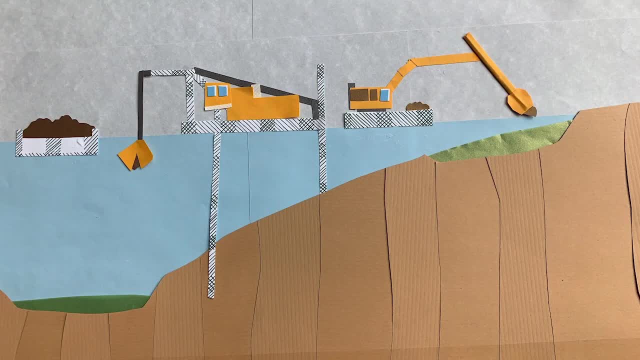 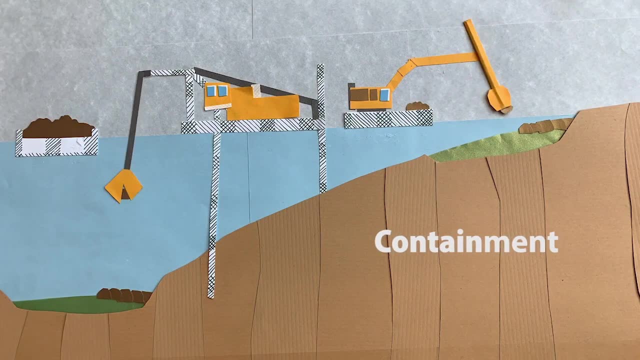 That's over 80,000 dump truck loads. In other areas, the plan calls for capping polluted sediment with clean sand Containment or capping covers the polluted sediment with a thick layer of clean natural materials, mostly silt, sand and rocks. 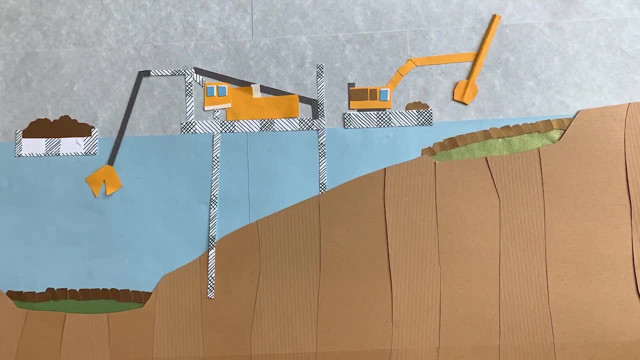 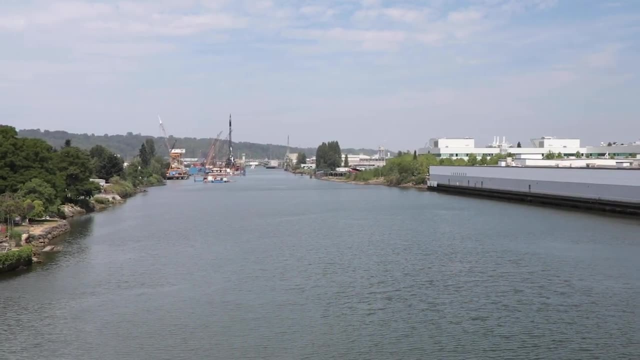 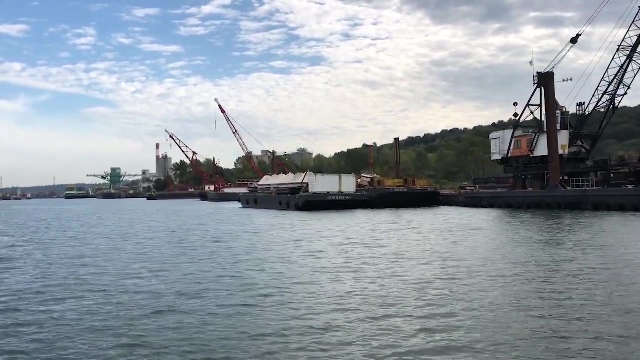 This is done in places where we are sure the cap will stay in place. In less polluted areas, we can allow natural recovery to occur as clean sediment drifts downstream from the Green River and settles in the Duwamish. And finally, in some areas we will need to speed up this natural recovery process by adding sand and potentially activated carbon. 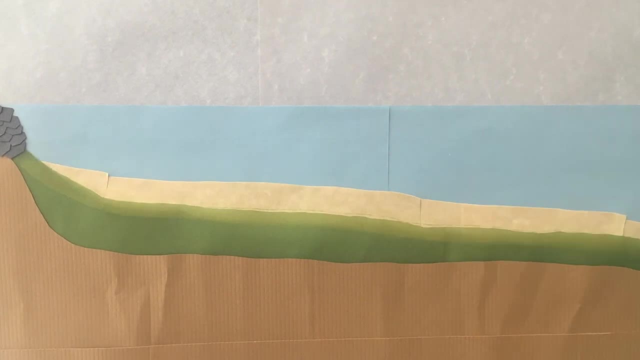 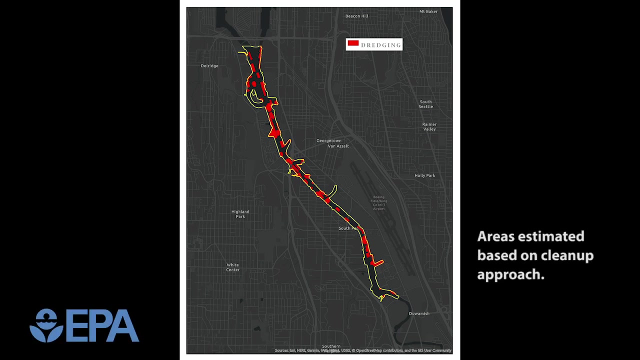 The kind you would find in a water filter. To give nature a head start, this approach is called enhanced natural recovery. EPA's cleanup plan estimates that about half of the waterway's 412 acres will be cleaned up with dredging, capping or enhanced natural recovery. 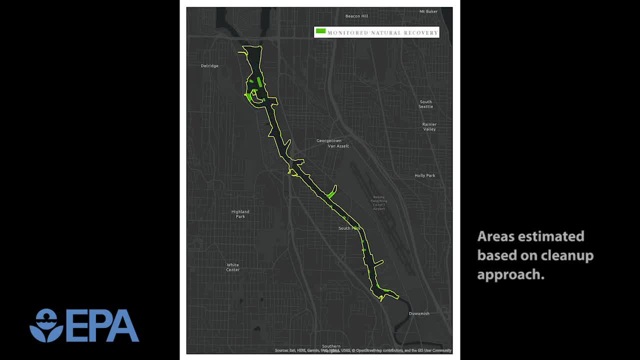 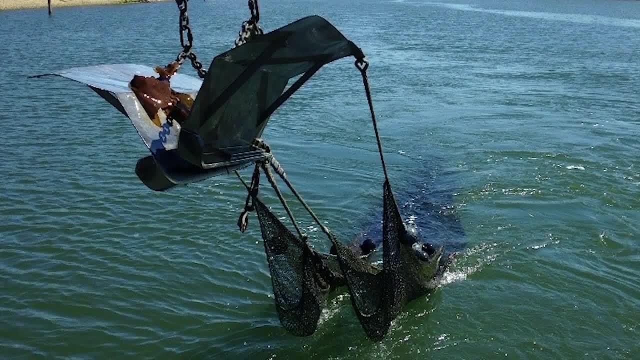 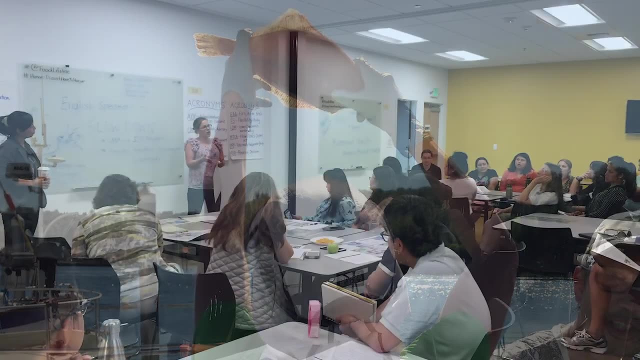 The remaining acres will be monitored as natural recovery processes continue the cleanup. Of course. this approach, like the others, requires close monitoring to ensure that it is working, Most importantly, to avoid having to redo cleanup. the work will go forward in stages to ensure that nearby sources of pollution are controlled. 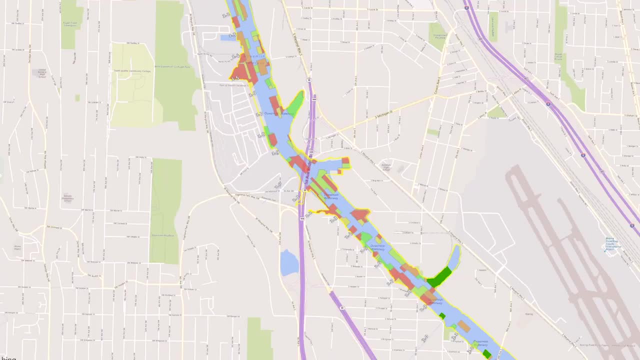 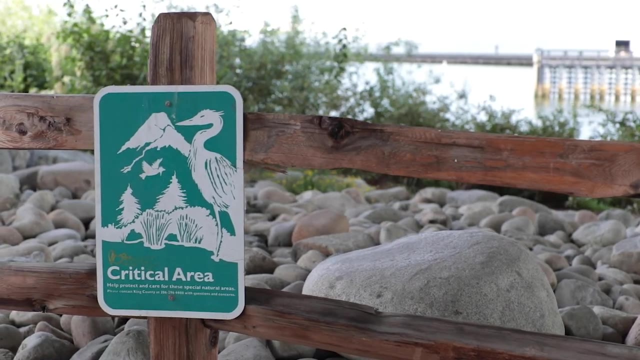 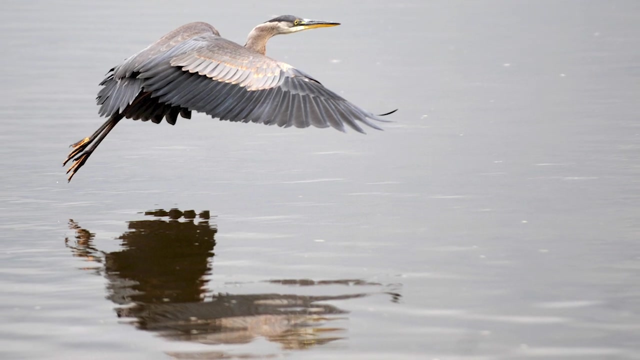 We anticipate three main stages of cleanup, starting with the most upstream two miles, called the upper reach. The cleanup is now getting ready for the design phase. Each phase of cleanup will require detailed engineering and monitoring plans. It's important to do the cleanup in a way that doesn't create new problems. 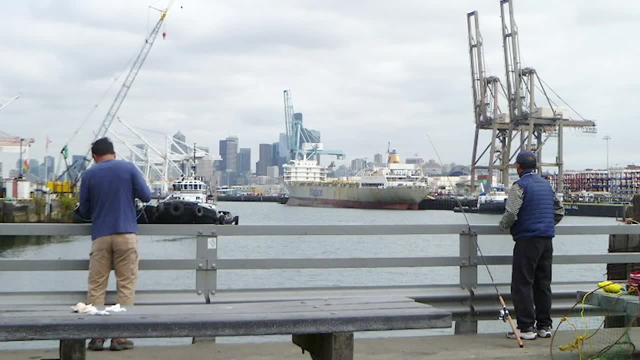 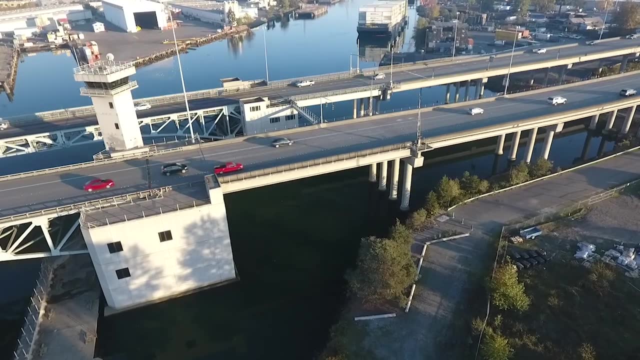 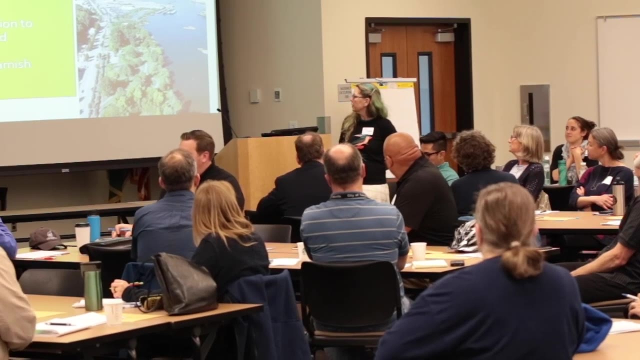 We want to make sure the cleanup restores the health of the river for the animals and people who live, work and play here, while keeping the river open for business. During the design phase, we will gather together community members, local agencies and other interested groups in the Duwamish Roundtable to help us minimize the impacts to the community and to make recommendations to improve the cleanup work. 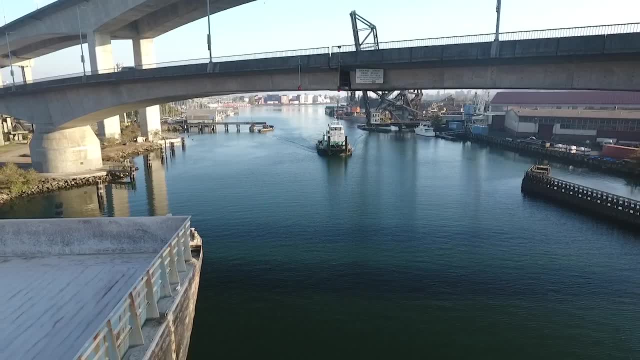 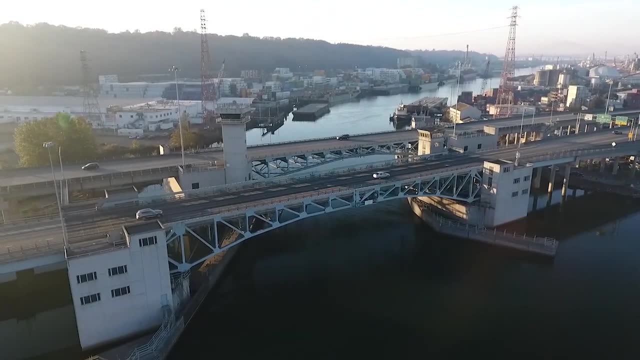 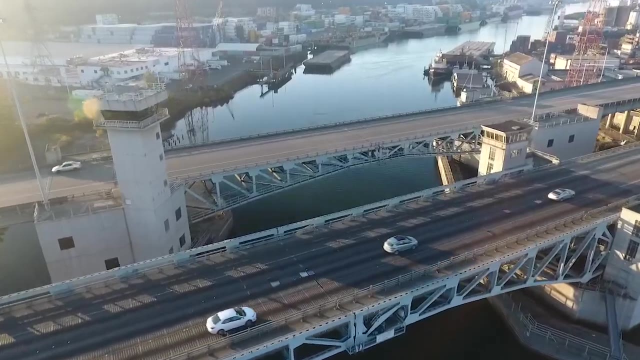 Once the upper reach design is done, cleanup will start. Design and cleanups of other sections will proceed down the Duwamish towards Harbor Island. The cleanup plan estimated that dredging, capping and enhanced natural recovery for the entire site would take about seven years once final plans are complete. Once active cleanup for all phases is done, we will monitor the areas to make sure that natural recovery continues to improve the river. With all this work, the cleanup plan is estimated to cost $342 million. The Lower Duwamish Waterway is an active waterway with commercial, industrial, residential and recreational uses on the water and shore. 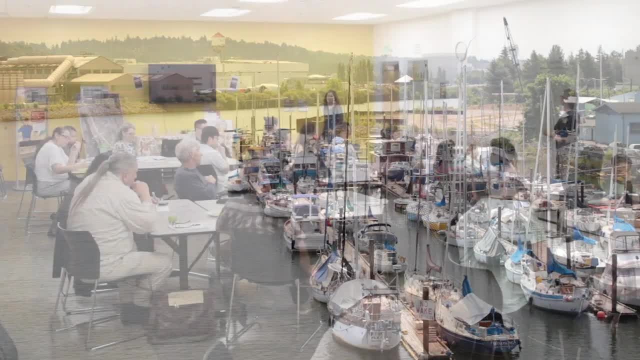 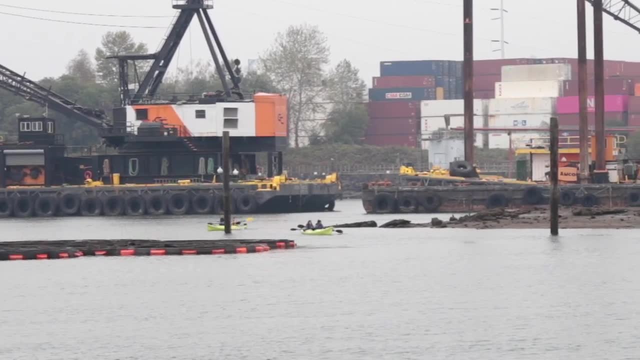 Many people live on the water in their boats. The come-in cleanup will take careful planning as the dredging and capping will take place in the midst of these ongoing uses of the waterway. As Seattle's only river, it's important to clean it up so that it can be a healthier river for generations to come. 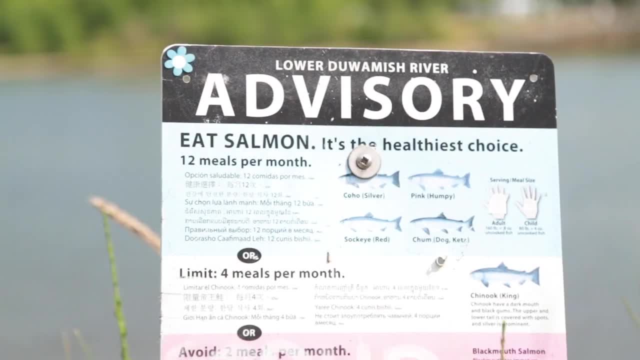 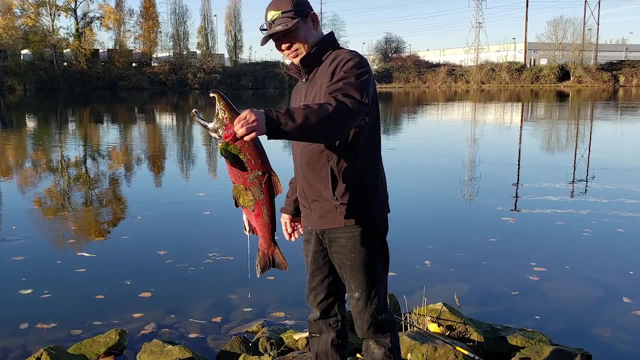 With so much information it can seem overwhelming, But here are some things you can do to contribute to a healthier Duwamish. If you eat fish from the Duwamish, only eat salmon. Salmon are in the Duwamish for only a short time of their lives and they are a safer choice to eat.